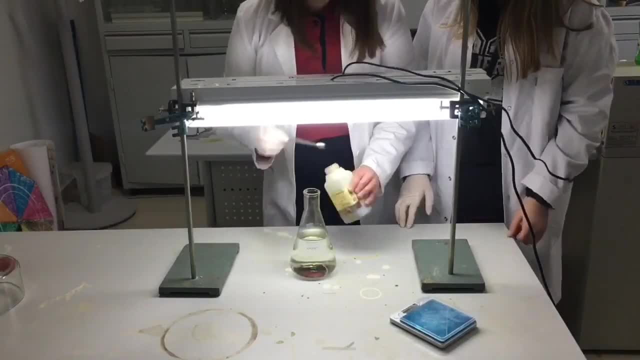 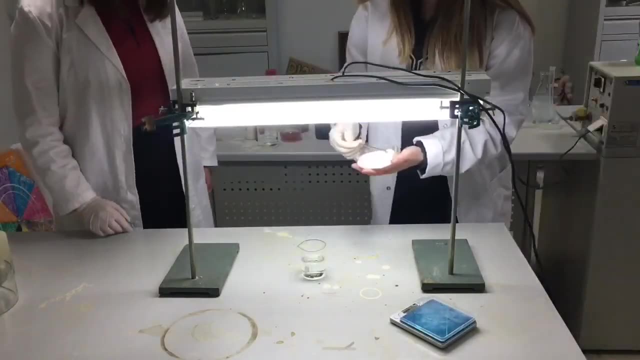 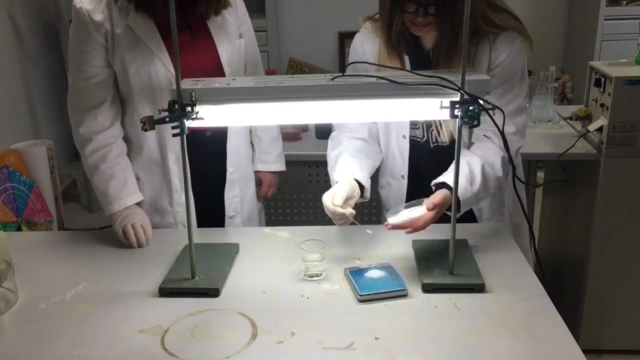 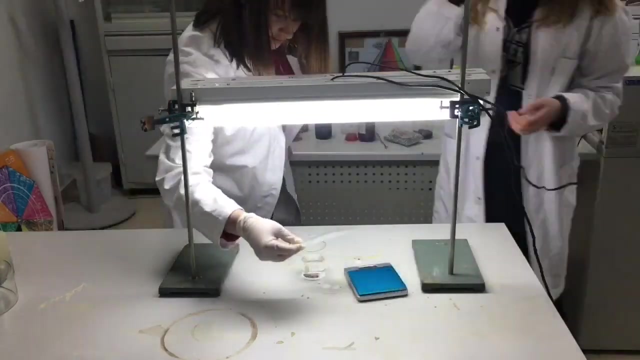 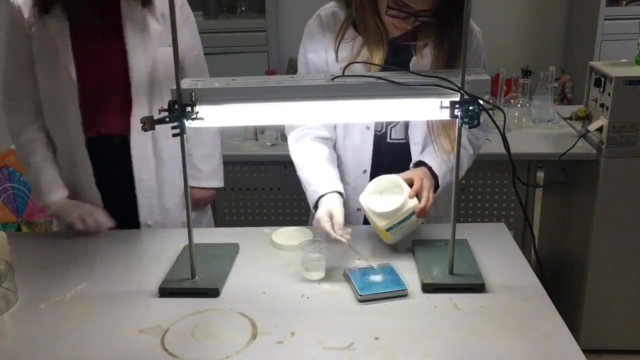 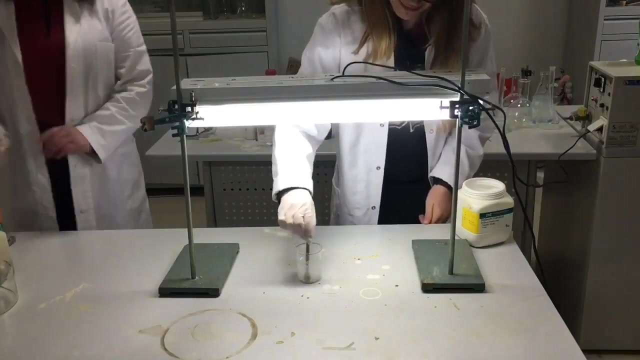 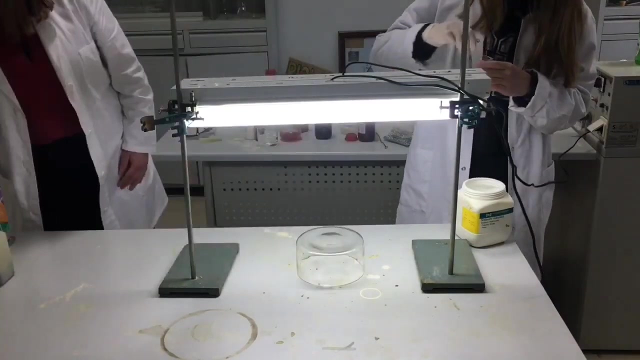 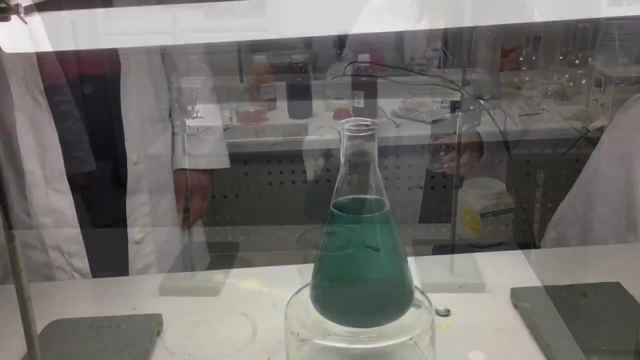 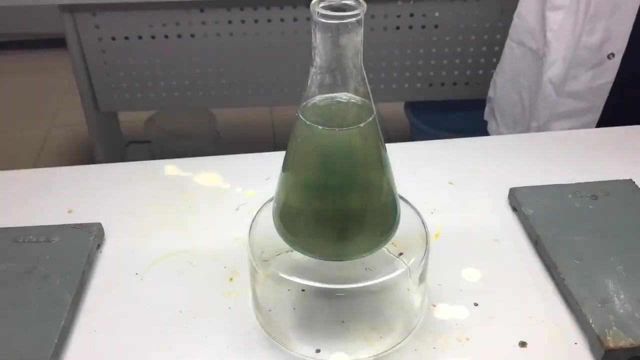 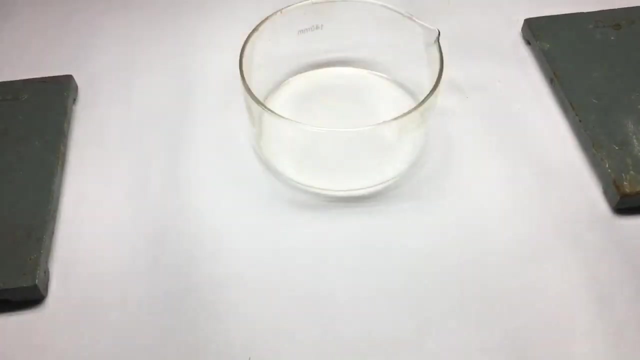 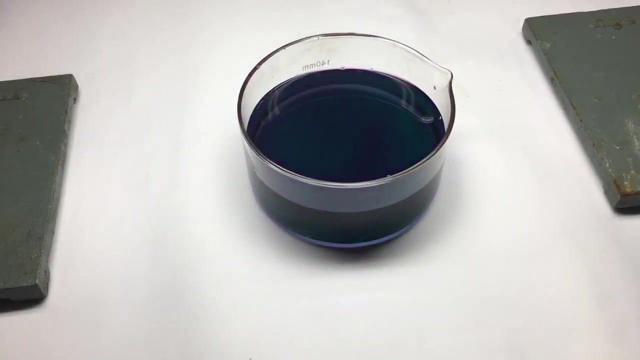 First we put potassium permanganate in the flask. Then we mix 2 grams of sugar with 1 gram sodium hydroxide and 75 ml of water. Now we mix the solutions together. Now we can see the purple color turning into green and then into orange. 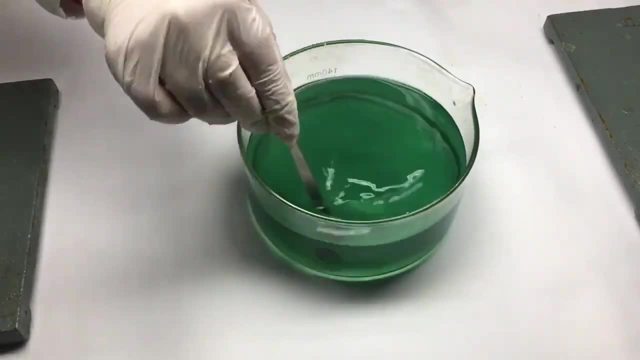 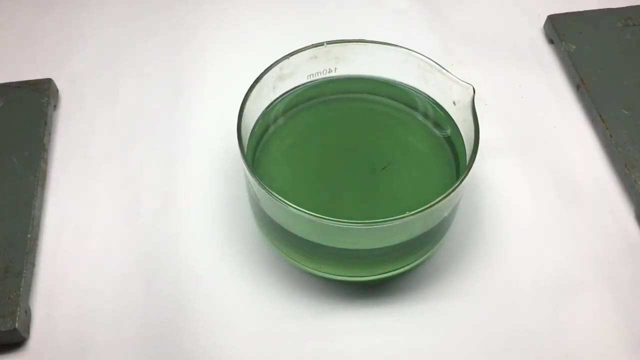 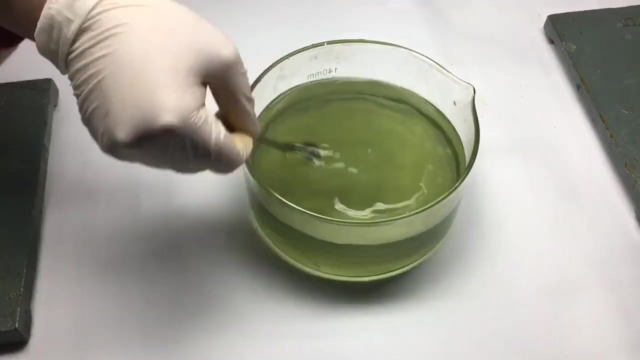 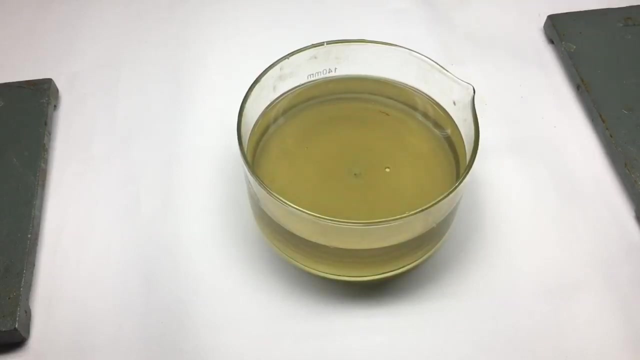 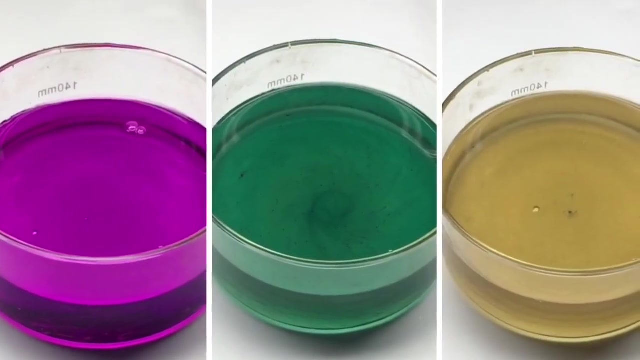 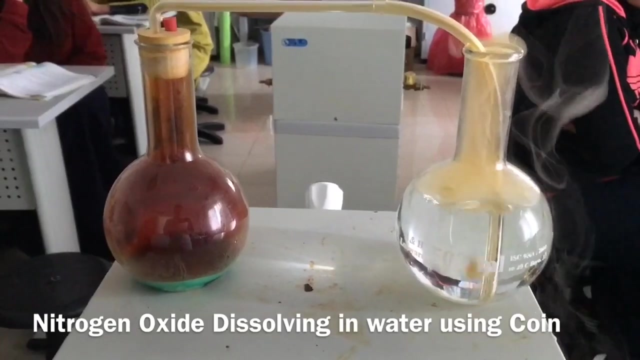 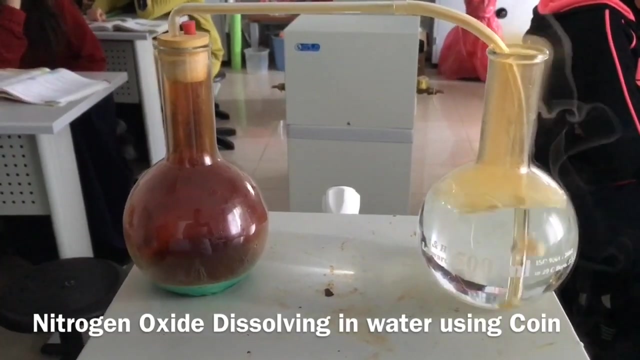 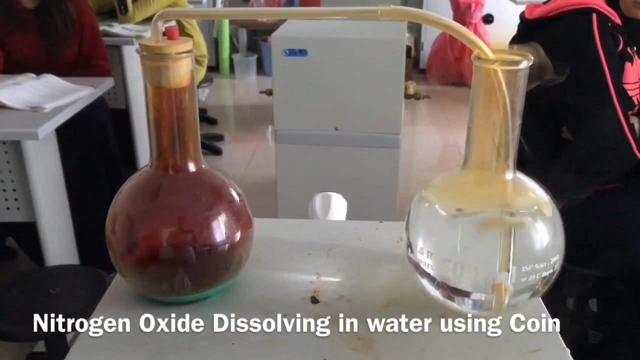 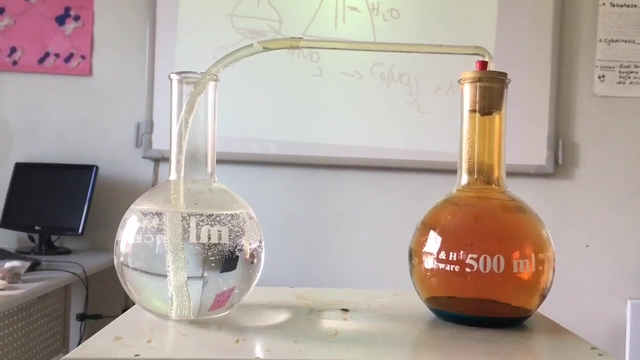 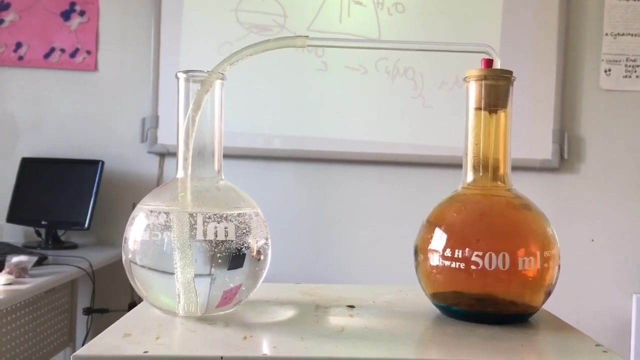 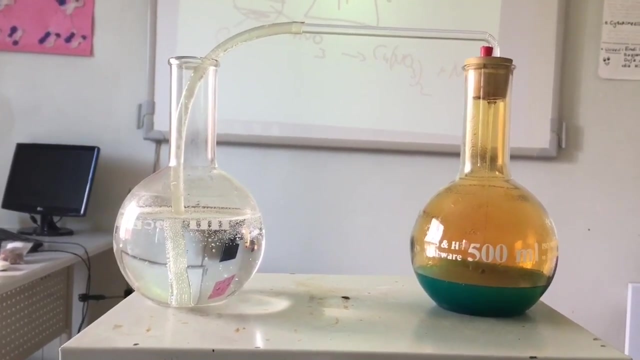 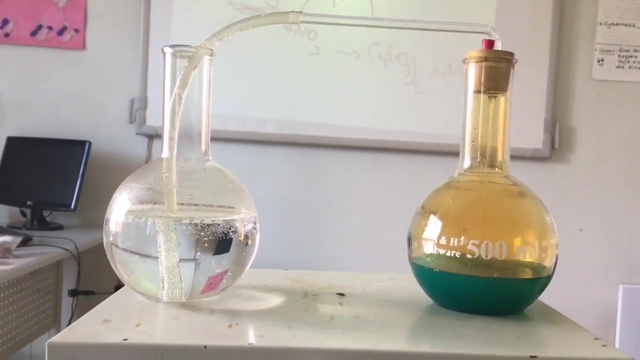 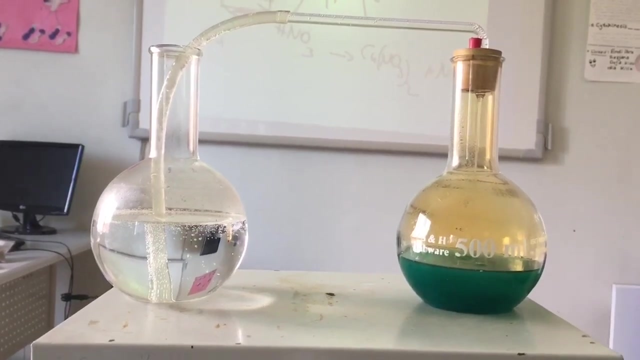 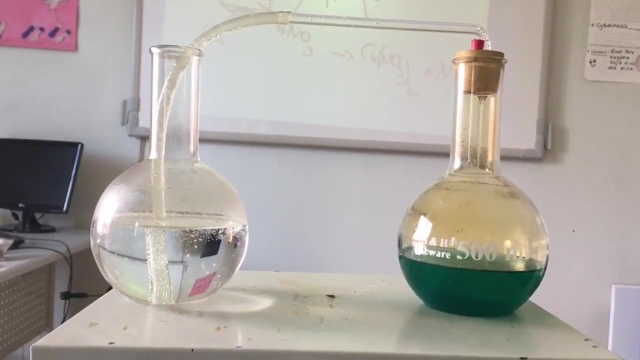 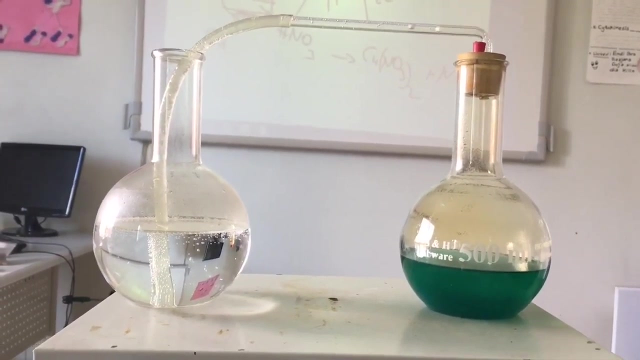 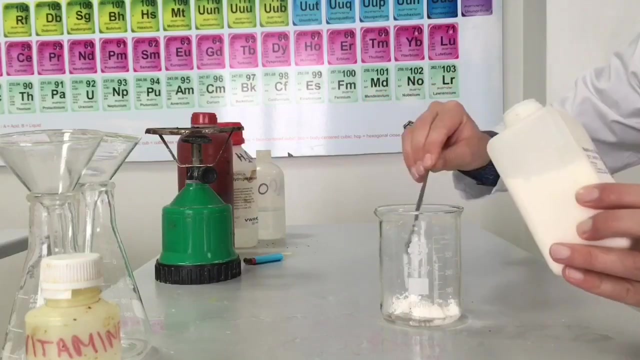 We mix it very carefully. As you can see, Clios is also very letzt. Now we pass it through another pot at a different temperature. 7 minutes, Thank you, Thank you. We are presenting you iodine clock reaction. First we prepare starch solution. 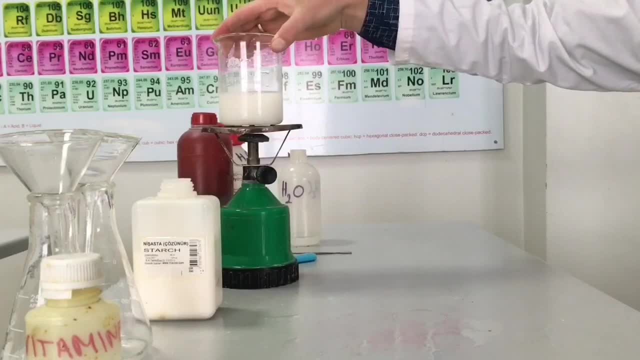 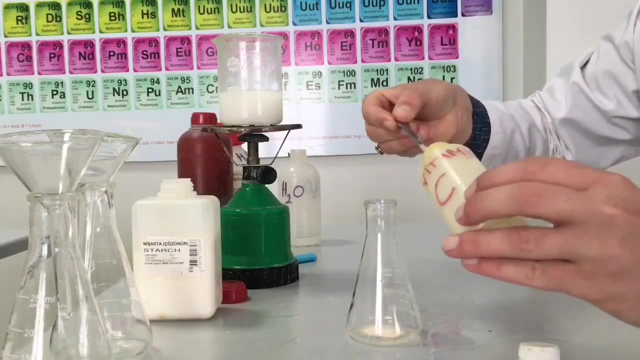 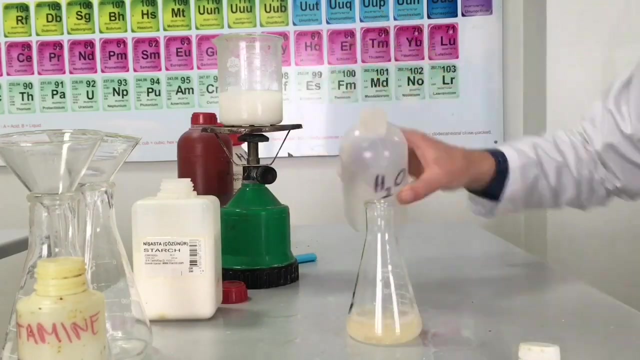 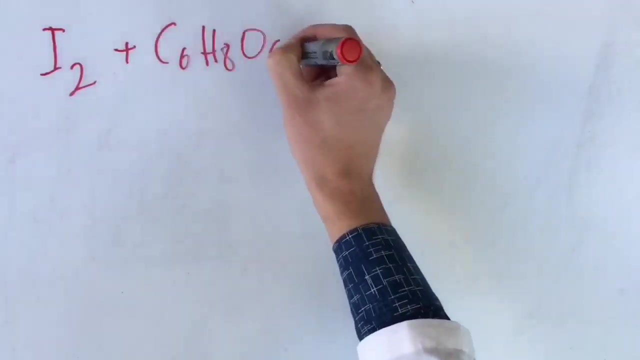 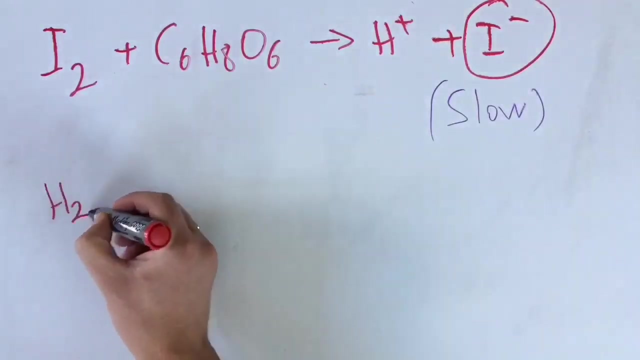 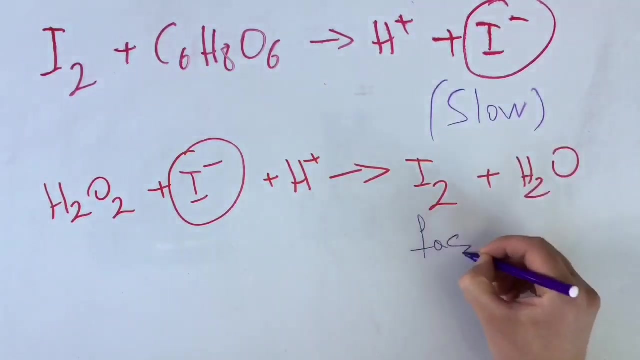 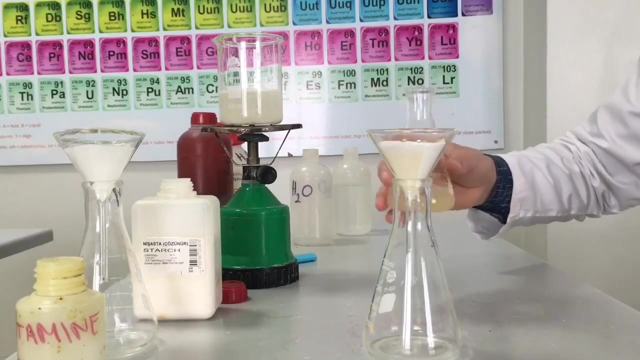 Now we are preparing C-vitamin solution. These two reactions are happening during the experiment. First of them is slow and the second is fast. So by this combination we can see the rate of reaction. We have to filter the solution of starch and the solution of vitamin C. 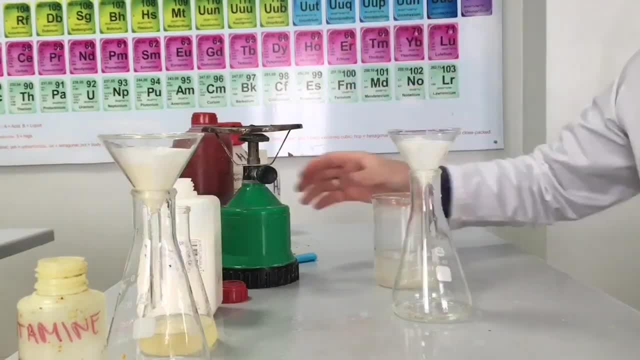 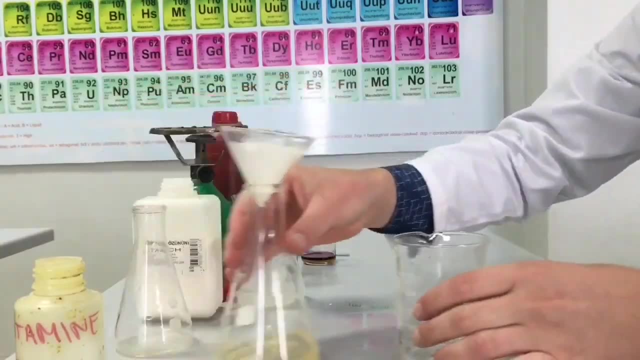 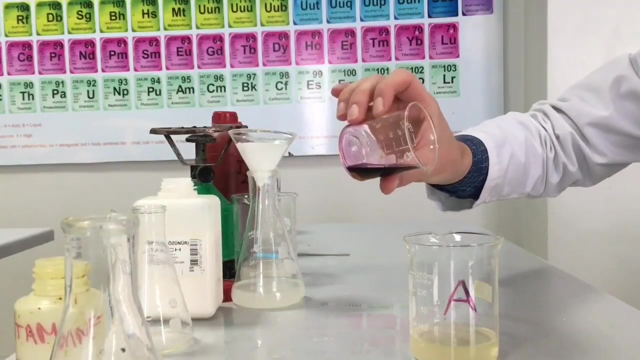 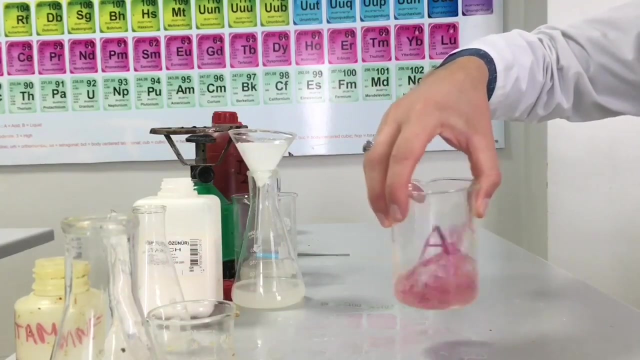 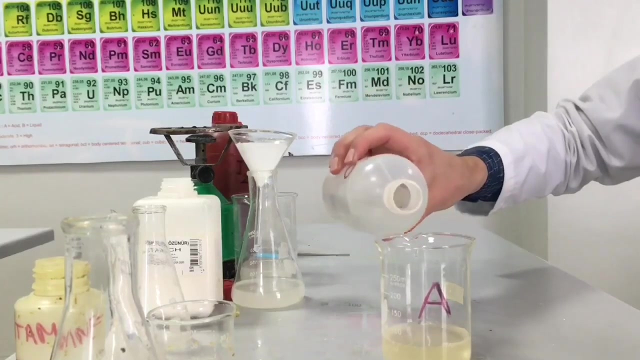 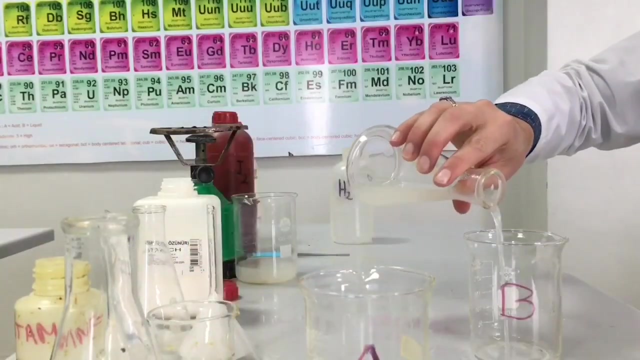 because we need a solution of vitamin C, And now we are preparing the colorless solution, And now we are preparing the solution A by adding the vitamin C and iodine. Solution B is prepared by adding starch solution and some quantity of 3% hydrogen peroxide. 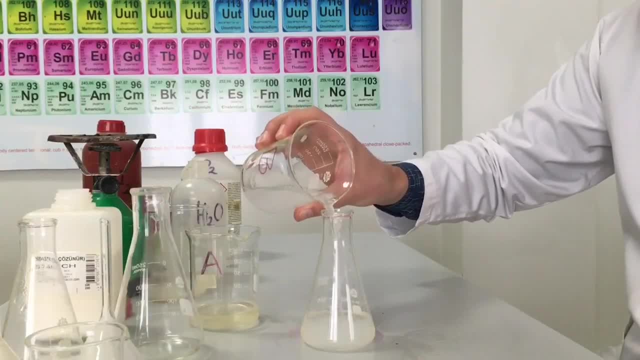 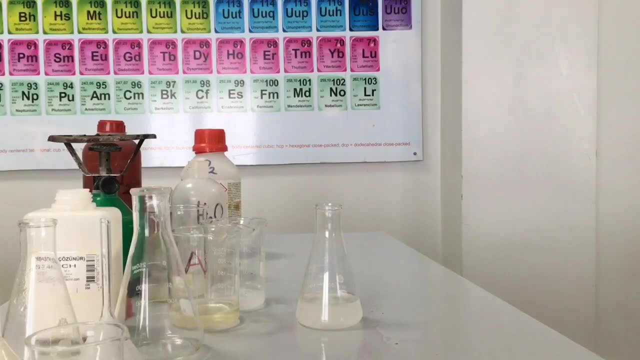 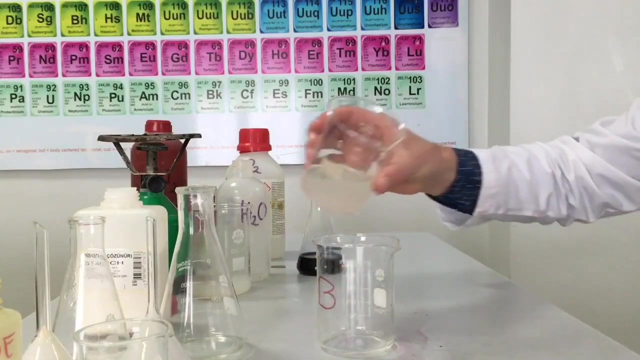 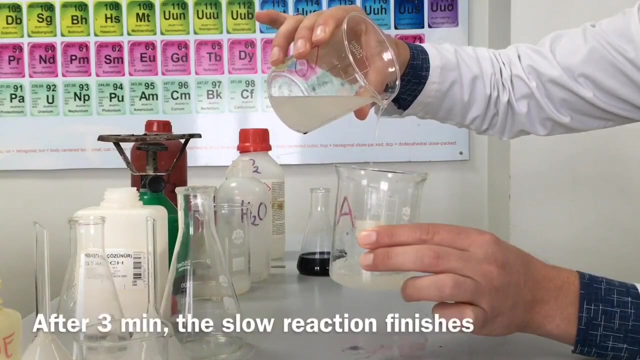 Here is final process, that mix in solution A and B. The blue dark color shows the presence of starch and the iodine. The blue dark color shows the presence of starch and the iodine. It means our solution. Then, familiar head refers to: 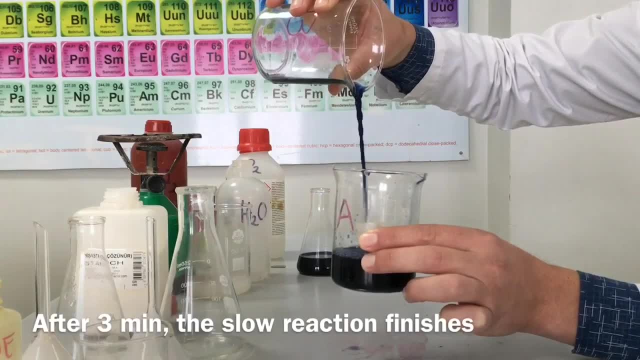 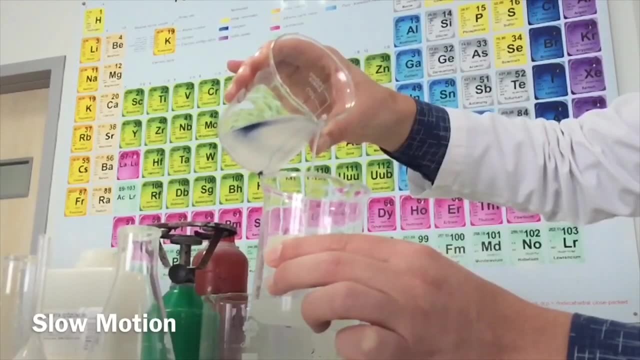 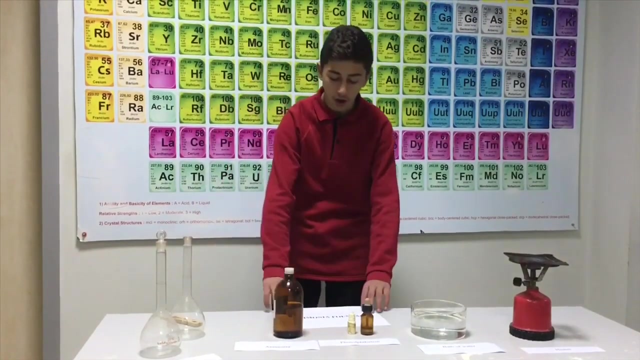 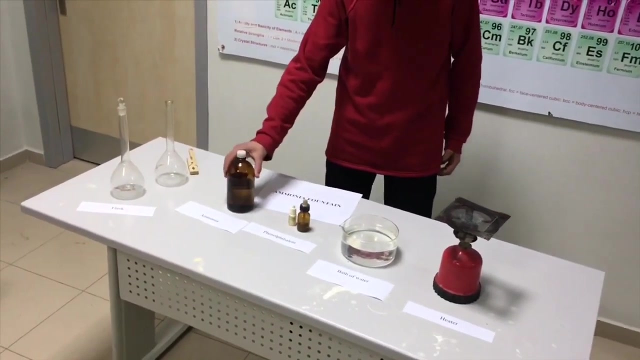 Since we add salt, the yellow color shows the presence of iodine. We add iodine to the solution when the color is white Water stop. Hello everyone. we are going to show you the experiment of Ammonia Falms. For this experiment we need a heater, a bath of water, phenolphthalein, ammonia and glass.